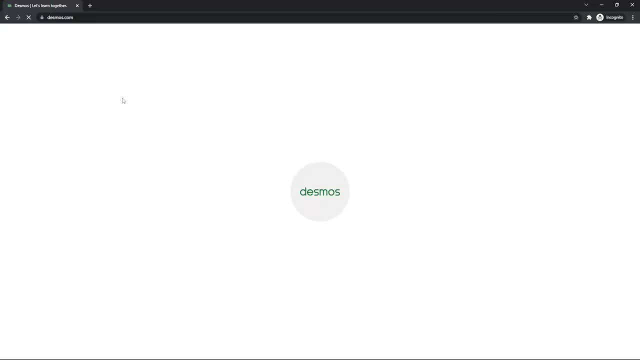 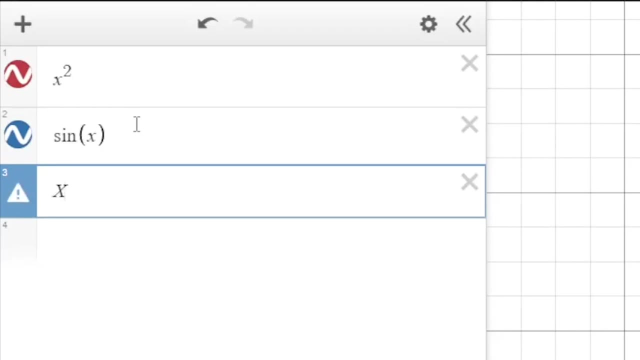 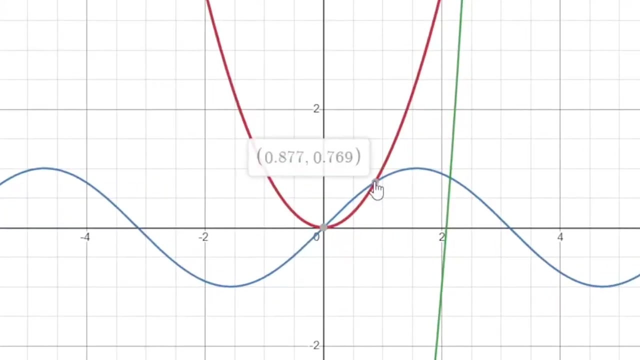 Desmos is a free online graphic calculator that students can use to graph functions, plot data and even evaluate questions. It lets you type in a function or multiple functions and it graphs those functions on the right. It's useful for when you want to visualize or calculate. 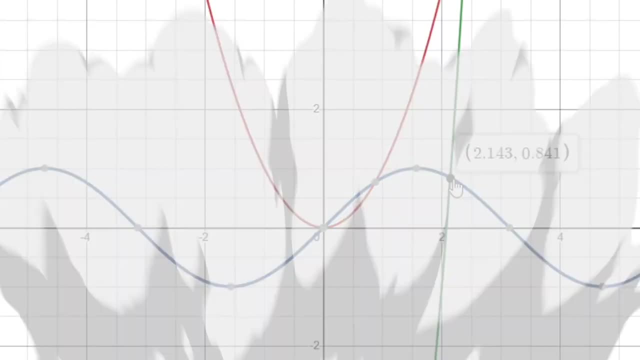 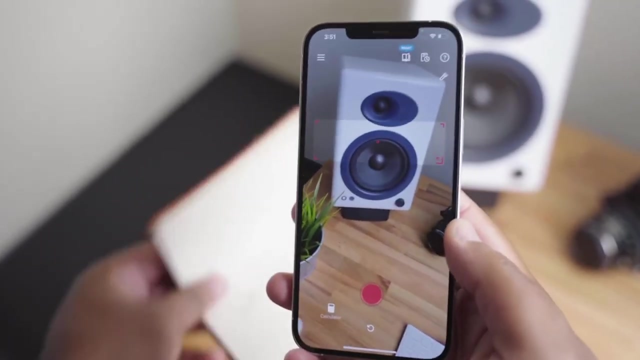 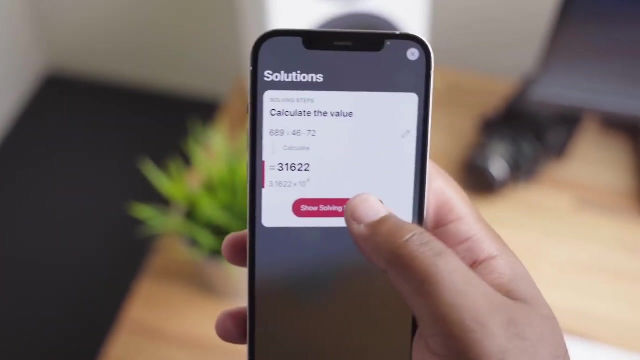 different equations that are hard to imagine on paper. Photomath is an app for your phone and it's good for solving math problems. You write down a problem on a piece of paper, take a photo of it and Photomath will show you step-by-step instructions of how to solve that problem. 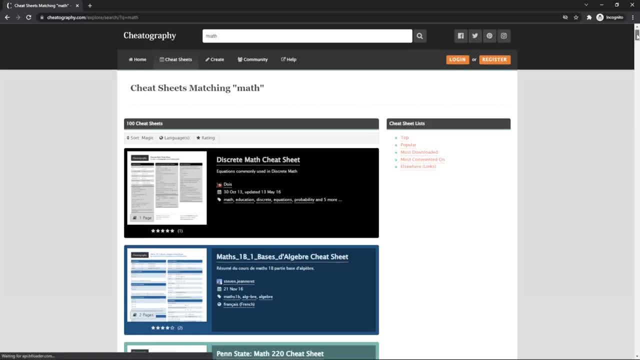 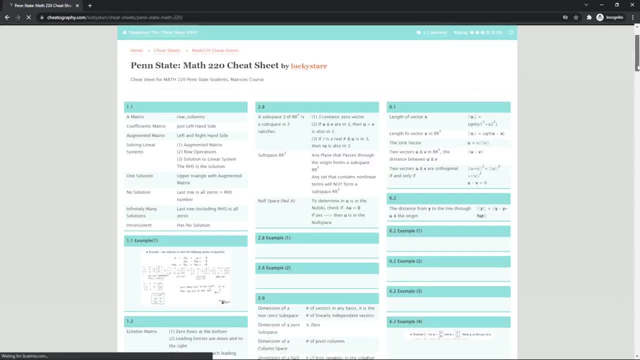 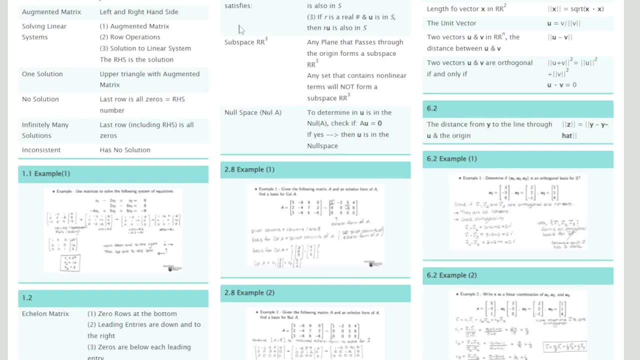 Cheatography is a collection of more than 4,000 cheat sheets and quick references in 25 languages for every subject, from history and math to French. You can choose your subject and discover handy revision aids and quick references, along with pictures of examples for your students to use in their classes. It's a great app for solving math problems. 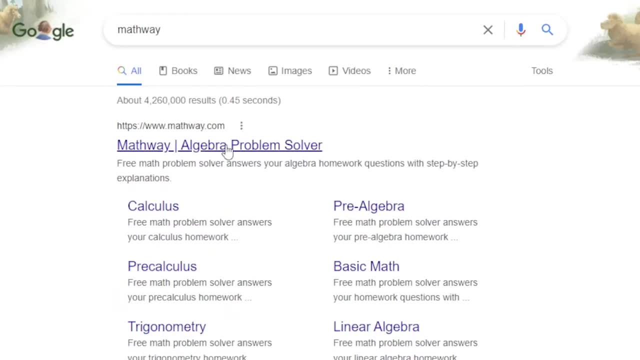 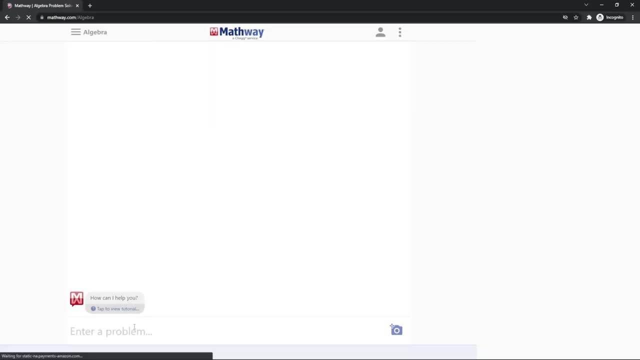 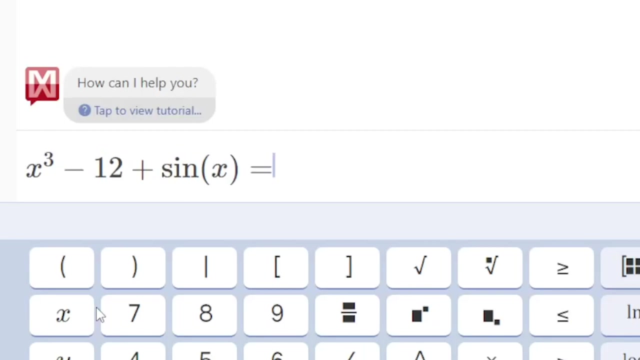 Mathway is another option for a free math problem solver that answers your algebra homework questions with step-by-step instructions. The website also offers an app that you can download and use to solve math problems on your phone. The app helps you with basically everything. 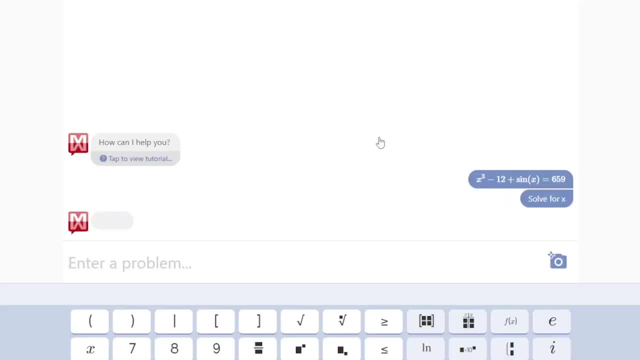 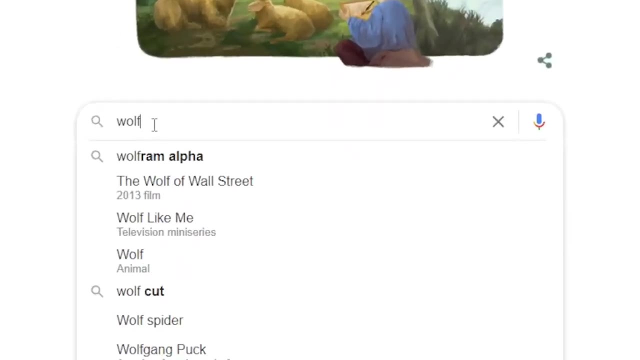 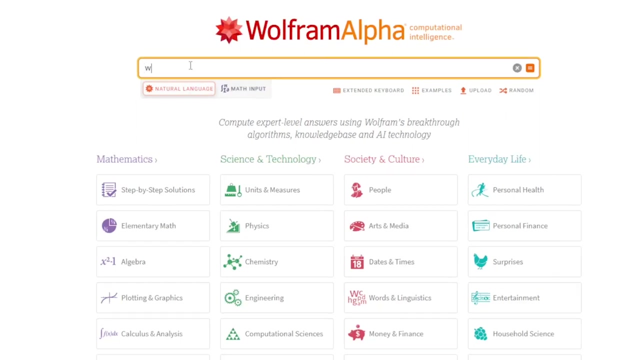 gives you answers and, if you don't want to fail a test, it even provides step-by-step explanations on how to solve your math problems. Wolfram Alpha is a unique engine for computing answers and providing knowledge. In simpler words, it helps you solve various problems related to math, science and even everyday life. It works. 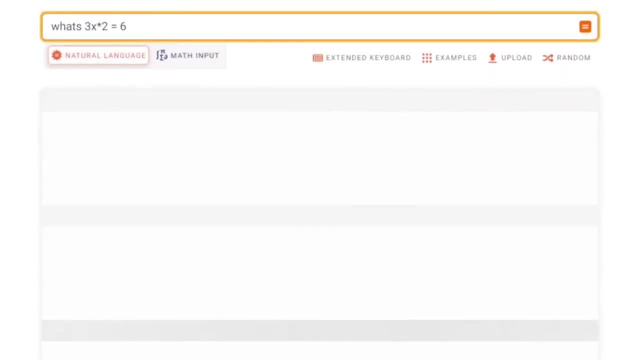 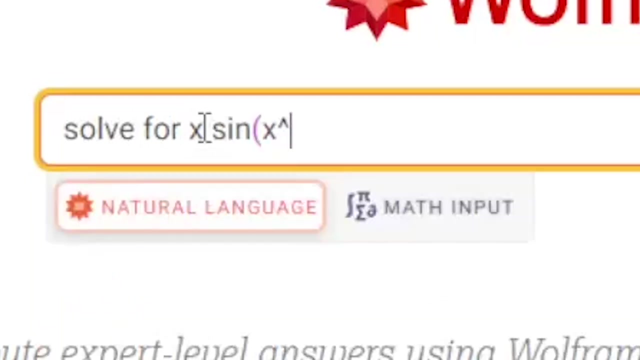 by using its vast store of knowledge and algorithms to automatically answer questions, do analysis and generate reports. So if you have a problem, you just type it in the search bar and the AI will solve it for you, as well as show you how to do it. 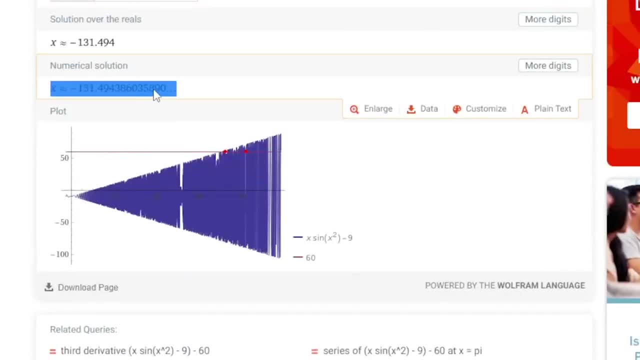 The website is surprisingly easy to use because in most cases, the search function interprets your natural language pretty well. This has been 5 websites that can help you with math homework, and if you liked what you saw in this video, consider watching the next one.